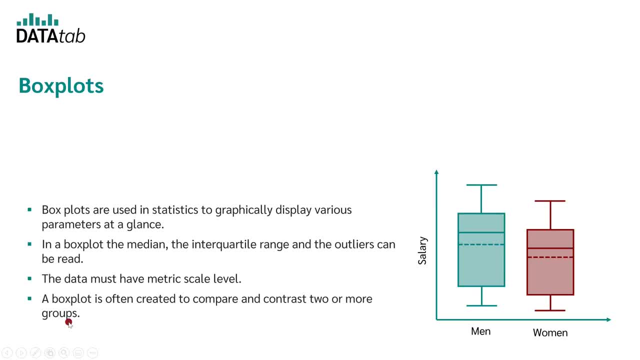 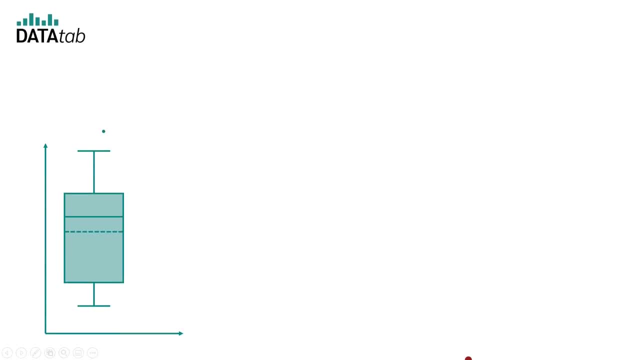 and contrast two or more groups, For example the salary of men and women. Now we'll look at what information we can find in a boxplot. Afterwards we'll go through what we've learned with an example. The box itself indicates the range in which the middle 50% of all values 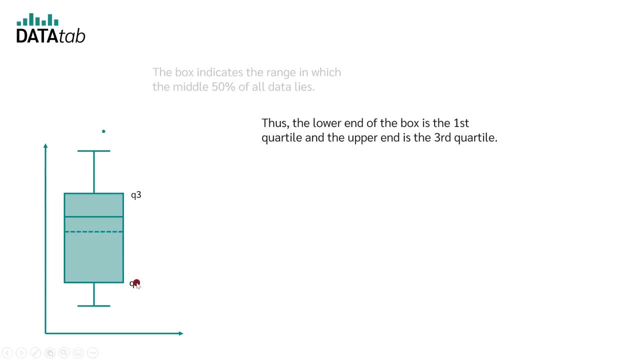 lie. Thus, the lower end of the box is the first quartile and the upper end is the third quartile. Therefore, 25% of your data are below Q1 and 25% of your data are above Q3.. Again in the box we find 50% of your data. Let's say we look at the age of people in a boxplot. 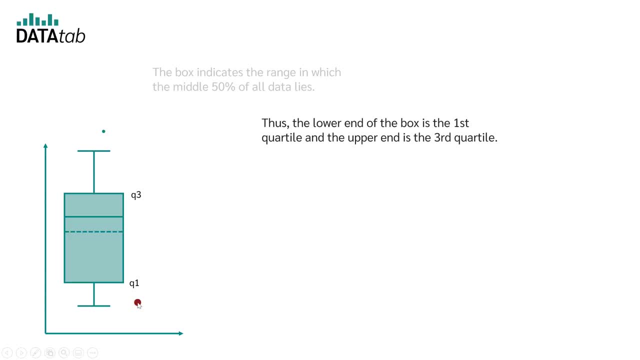 and Q1 is, let's say, 19 years, This means that 25% of the participants are younger than 19 years. if let's say Q3 is 55 years, This means that 25% of the participants are older than 55 years. 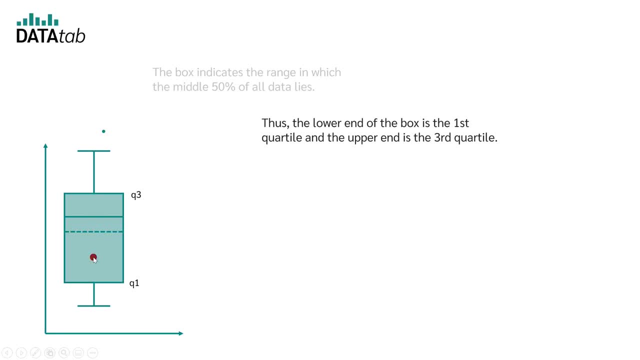 And 50% of your participants are therefore between 19 and 55 years old. Between Q1 and Q3, we have the so-called interquartile range. In the boxplot, the solid line indicates the median and the dashed line indicates the mean. For example, if the median is 34, this would mean 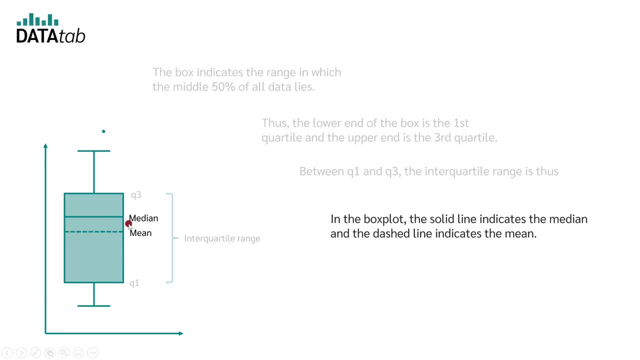 that half of the respondents are younger than 34 years old and the other half is older than 34 years. The median thus divides the individuals into two equal groups. Further, we have the T-shaped whiskers. The T-shaped whiskers indicate the last point, which is still within 1.5 times. 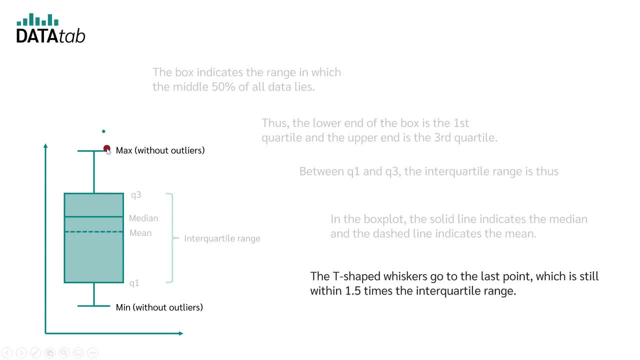 the interquartile range. What does that mean? Here we can see the interquartile range. The T-shaped whisker is either the maximum value of your data, but at most 1.5 times the interquartile range. Therefore, 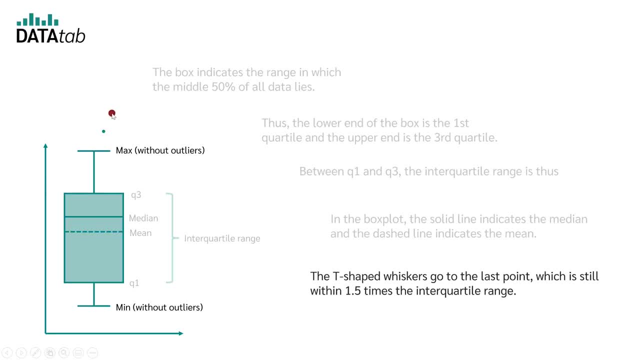 if you have an outlier, the T-shaped whisker goes up to 1.5 times the interquartile range. If there is no outlier, the whisker is the maximum value. The same is true for the lower whisker, which is either the minimum value or 1.5 times the interquartile range. Points that. 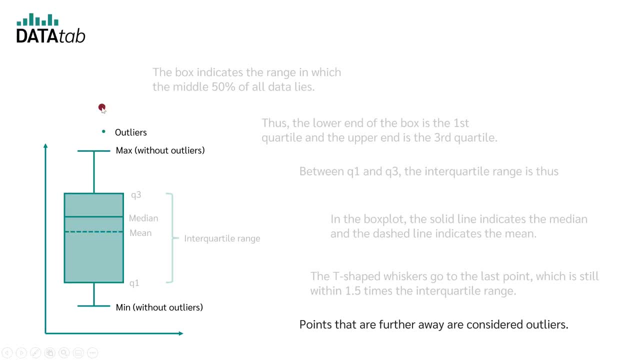 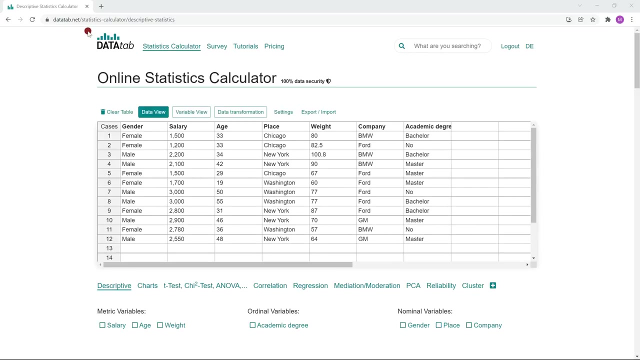 are further out are considered as T-shaped whiskers Outliers If no point lies further out than 1.5 times the interquartile range. the T-shaped whisker indicates the maximum or minimum values. So, and now we will look at an example. In order to do this, we will go to datadepnet. 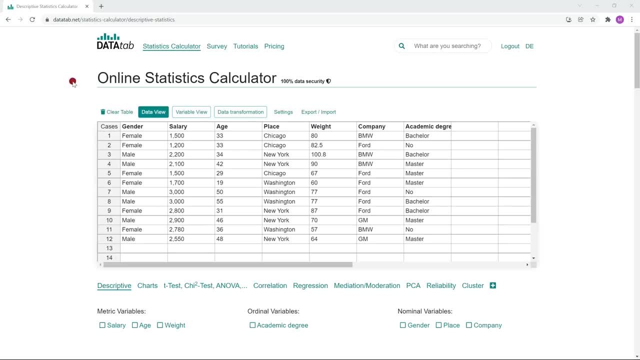 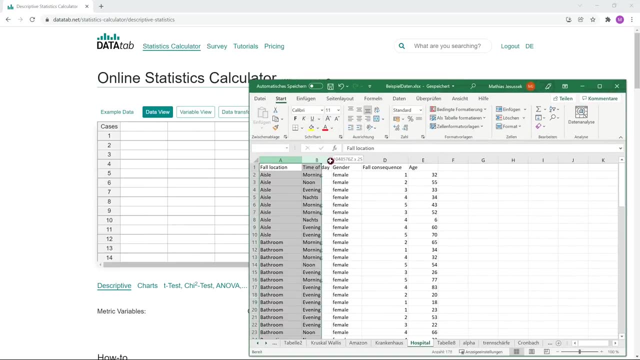 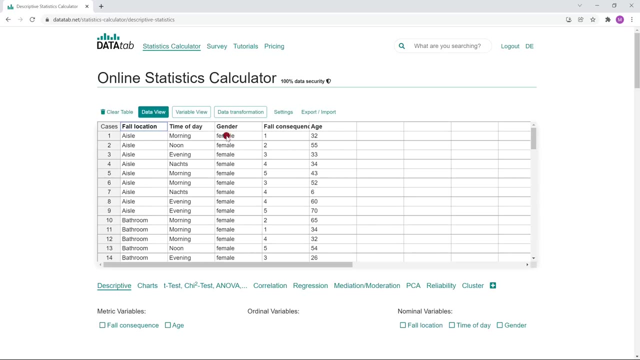 You will find the link in the video description And then we copy our data into this table. This is a correct graph. You will find a tom períikum for the unit of dose. Here we have a dataset where every fall of a patient in a hospital was documented. 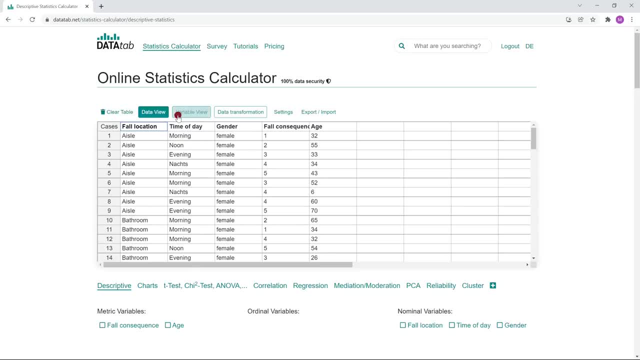 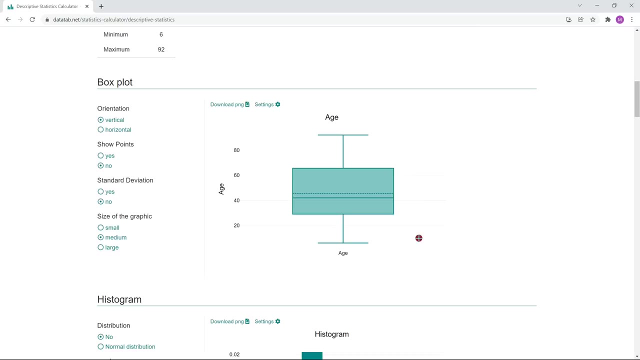 After each fall, we asked where the fall occurred, At what time of the day it happened, what gender the person had, what the consequences of the fall were And, finally, the age of the person. If we now click on Age, get the boxplot for age, We see that the maximum value is 92 years and the minimum value is 6. 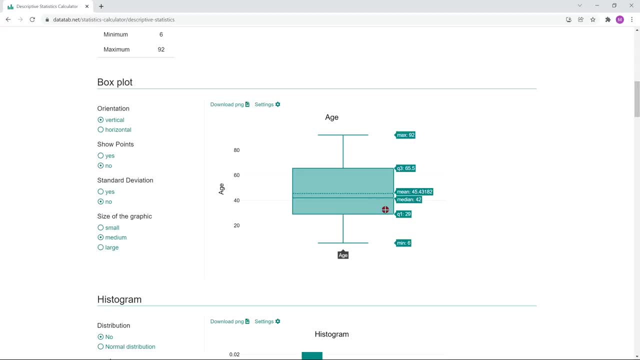 years. Q1 is 29 years, So between 6 and 29 years, there are 25% of the people, And between 29 and 65.5 years, there are 50% of the people. Then between 65.5 and 92, there are the top 25%. 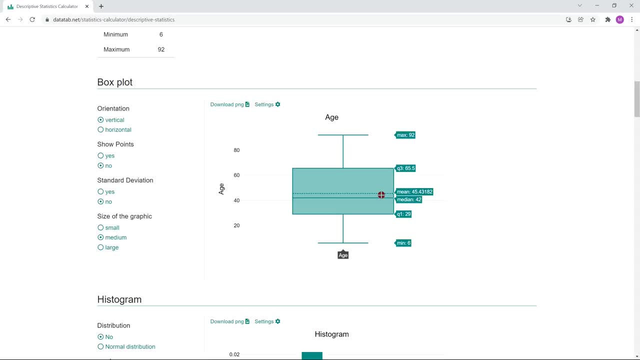 We can also see that the mean is 45.43 and we have a median which is 42. So half of the fallen people are younger than 42. And the other half are younger than 42. And the other half are younger. half is over than 42. If you like, you can change the direction here and you can see all the points.